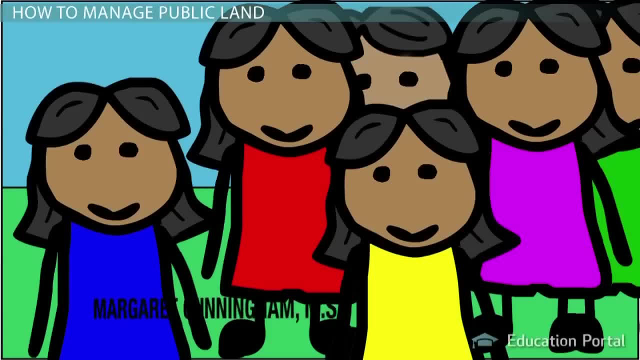 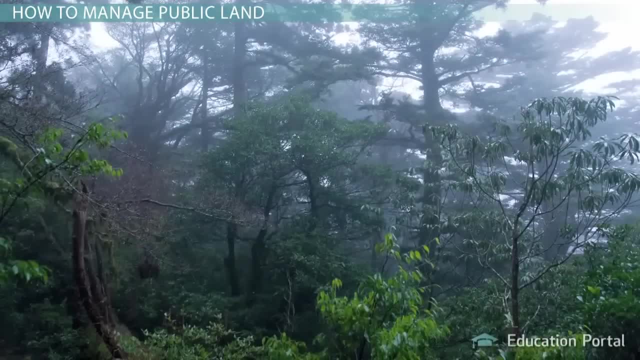 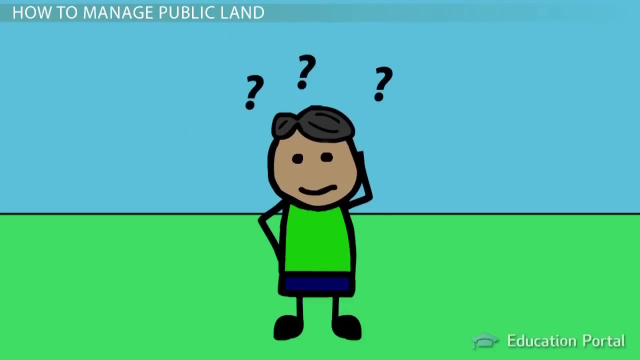 As the human population grows and grows, natural resources are being used at a rapid rate and large areas of forest are being converted for human use. How do you think public land should be managed to deal with these types of environmental issues? Over the years, there have been many opinions on how to manage public lands. Two of the 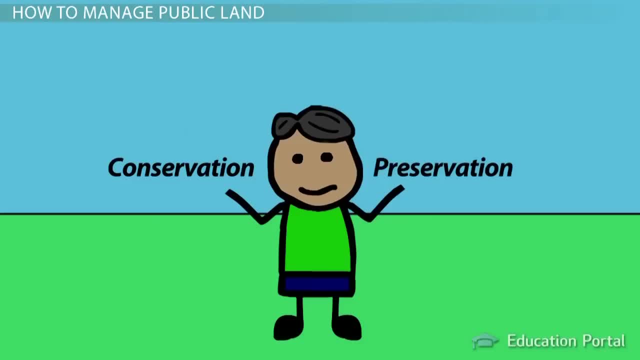 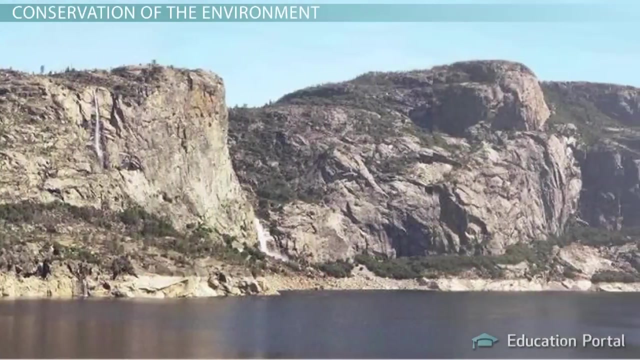 major points of view include conservation and preservation of the environment. People often use these two terms interchangeably when in fact they are two very different views and methods for managing land. Let's explore these two terms and how they vary from one another. Some people believe that public land should be managed by the method of conservation. 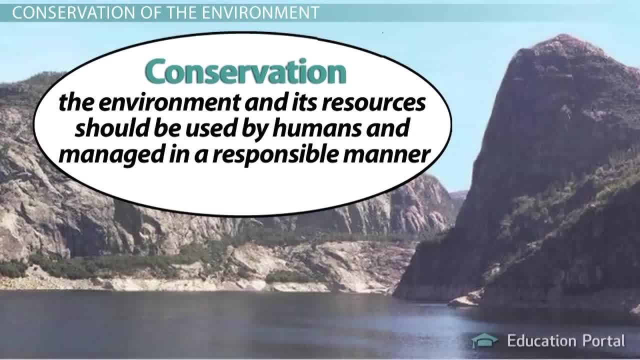 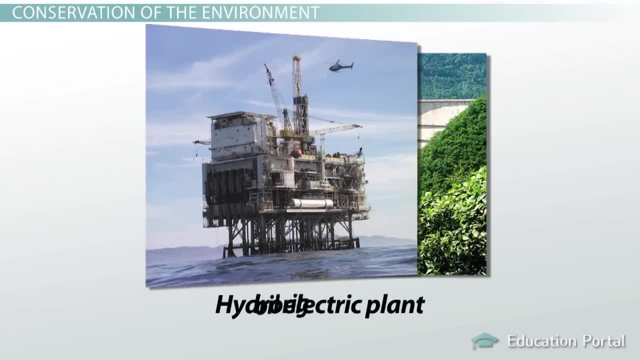 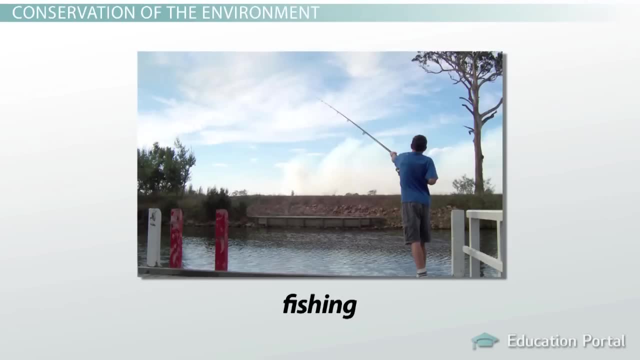 meaning that the environment and its resources should be used by humans and managed in a responsible manner. These types of people see the value of the environment as the goods and services that it can provide to people. This viewpoint requires that the environment be used in a way that is sustainable and ensures. 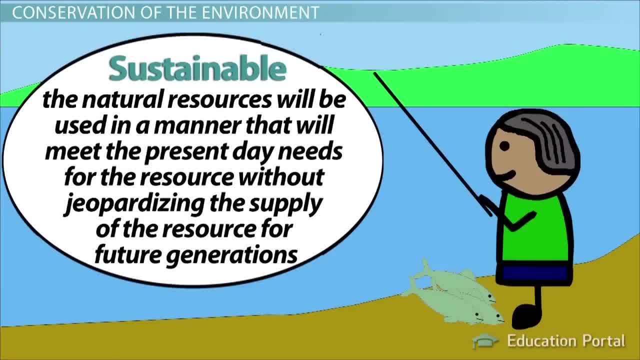 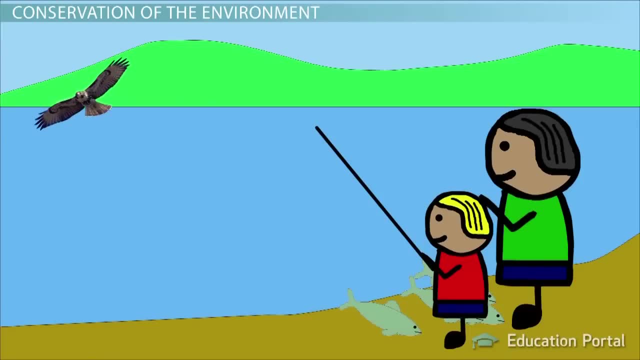 that the natural resources will be used in a manner that will meet the present-day needs for the resource without jeopardizing the supply of the resource for future generations. By using the environment sustainably, the environment and the natural resources it provides will not be depleted or destroyed permanently and will be available for human use for a. 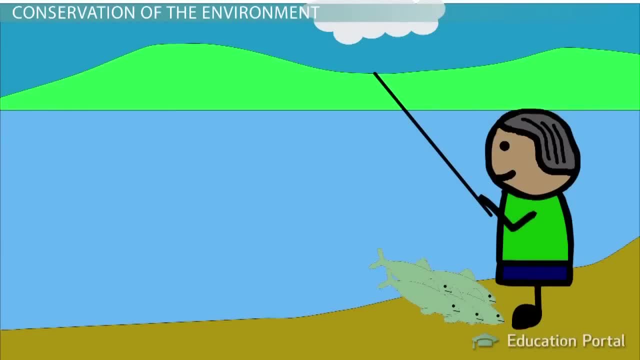 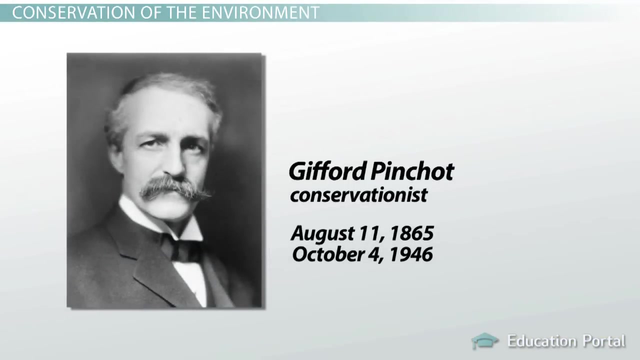 very long time. If people do not manage the land properly and the resources are not being used sustainably, then the environment can be destroyed and the conservation method will have failed. Gifford Pinchot, who lived from 1865 to 1946, was a leader in the conservation movement. 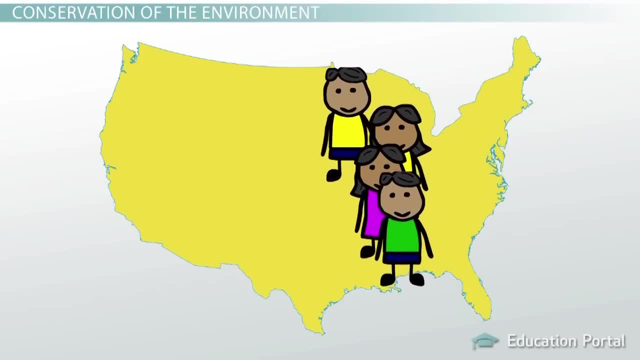 As the United States expanded and more land was being converted for human use, Pinchot was bothered by the method used in transforming the environment. Pinchot, who lived from 1865 to 1946, was a leader in the conservation movement As 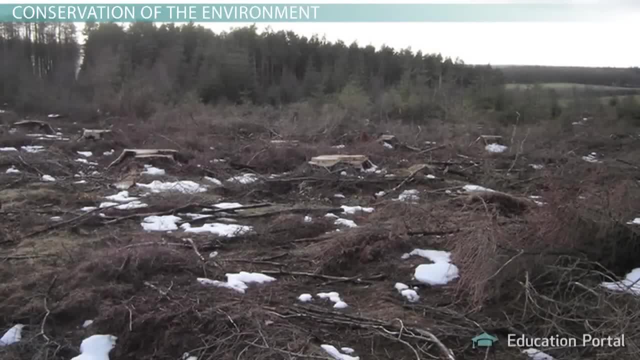 the United States expanded and more land was being converted for human use. Pinchot was bothered by the method used in transforming the environment. At the time, most forests were being clear-cut, which is when all of the trees are removed at the same time. Pinchot did not like this method because he saw the forests as a valuable 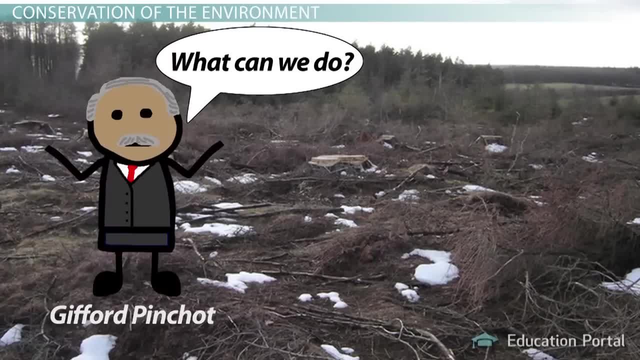 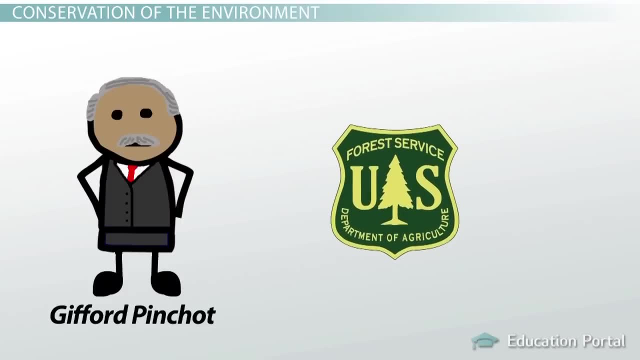 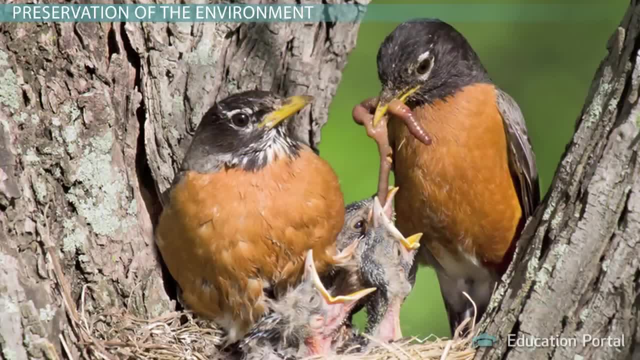 He later founded the organization that would become the US Forest Service and served as chief of the organization, while theorizing about the use of natural resources, protection of land, and believe that people should only use the environment for enjoyment and not as a resource for goods. 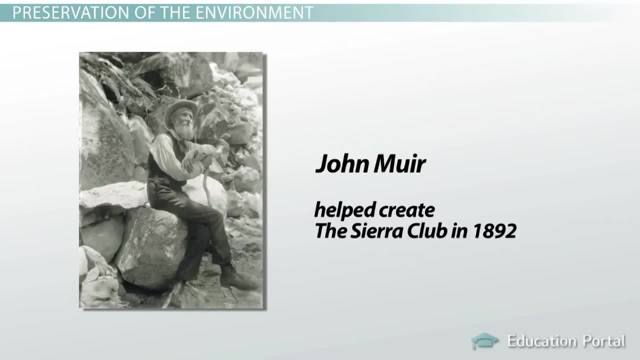 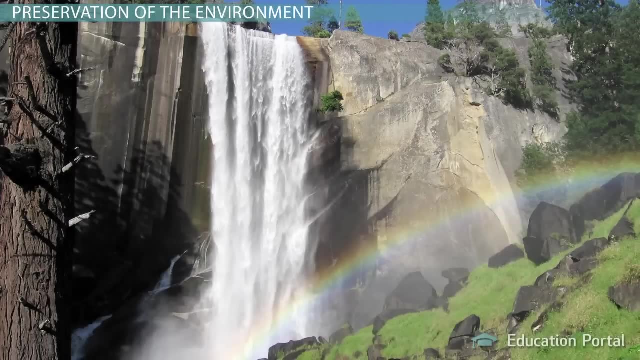 Muir was involved in the creation of the Sierra Club in 1892, which is an environmental organization that advocates for the preservation and protection of public lands.